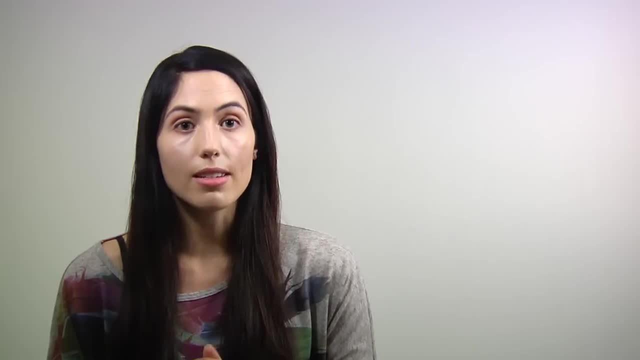 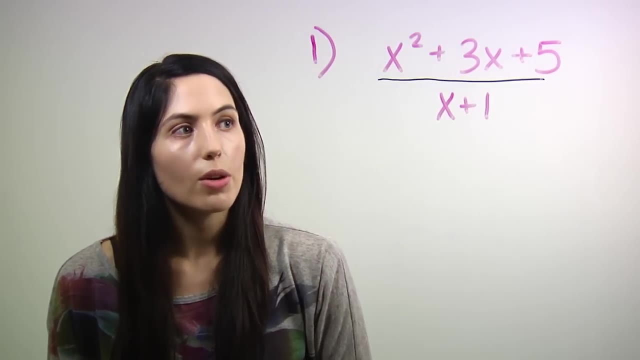 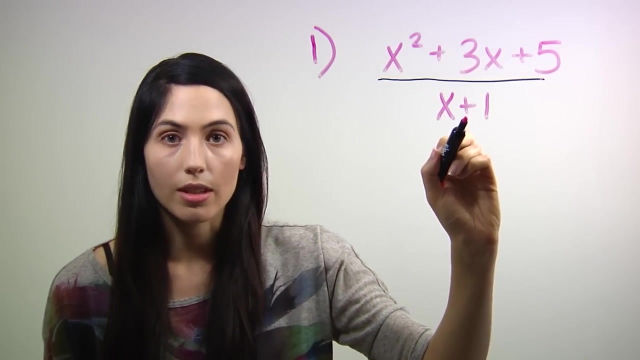 it's come back to haunt you in high school. So let's look at a simple example first. Okay, so you've been given a rational expression, that is, one polynomial divided by another polynomial, and now you need to use long division. So the first thing you need to do is rewrite. 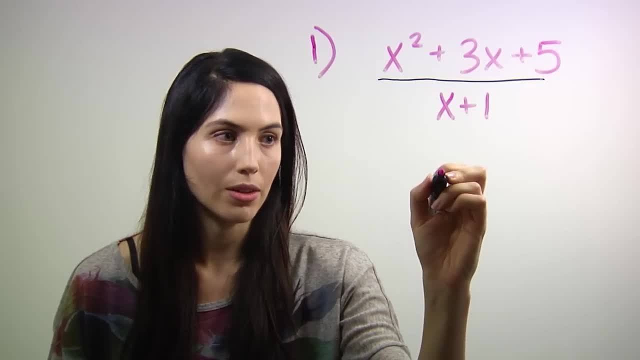 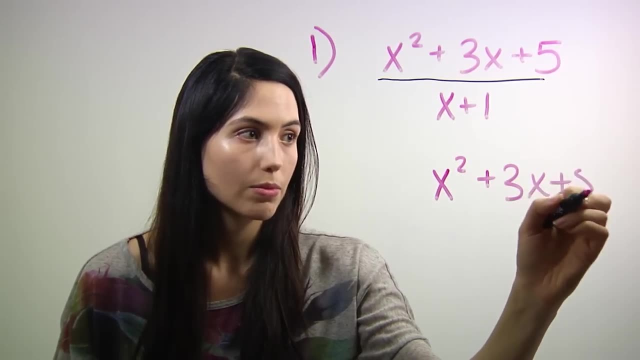 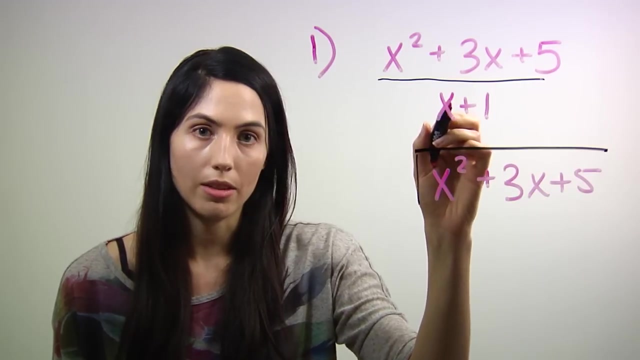 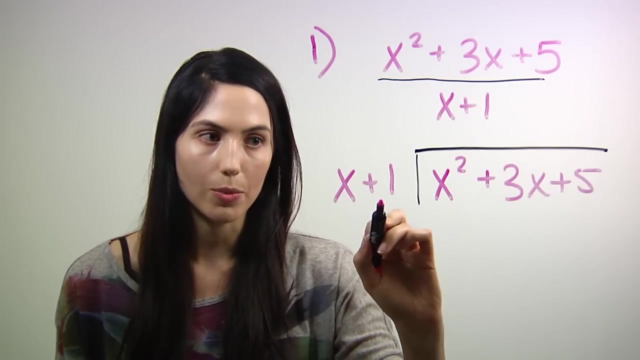 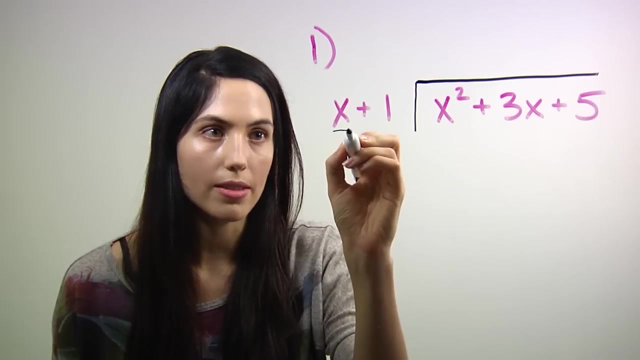 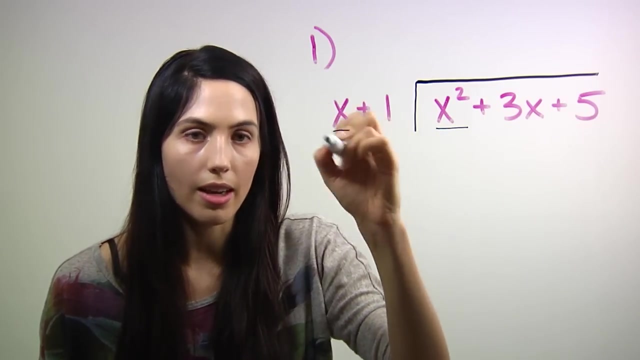 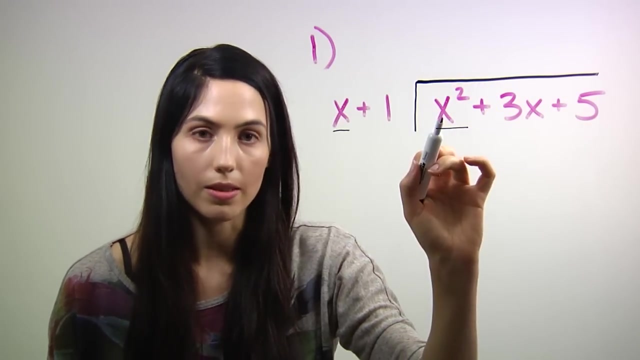 this rational expression in the old division form that you're used to from elementary school. So the top polynomial goes underneath the division sign and the bottom polynomial goes to the left. So this still means x squared plus 3x plus 5 divided by x plus 1.. Okay, so the first step is to look for the highest power of x on this side and the highest power of x on this side and find how many times does this x go into that x squared, and that's x times, since x times x gives you x squared. 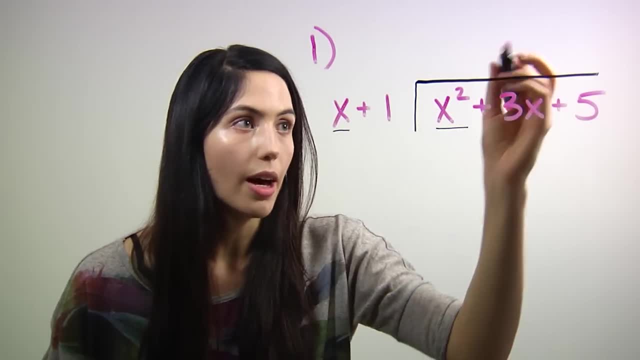 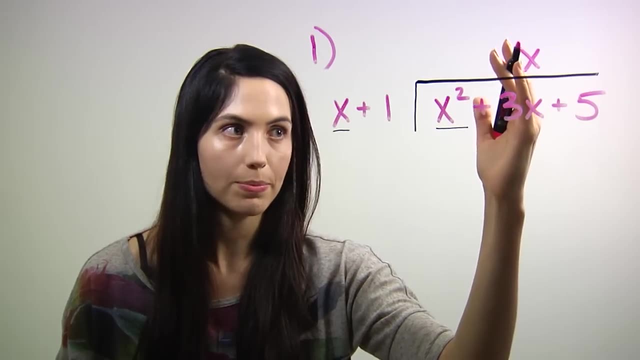 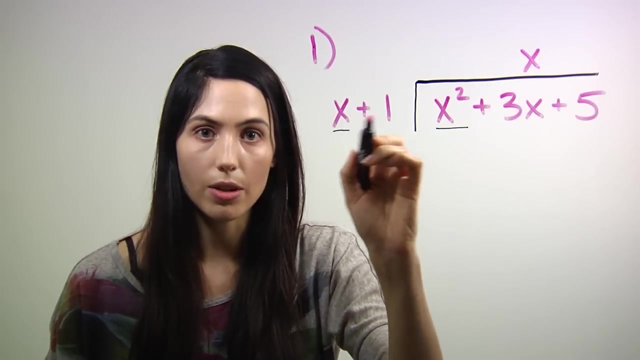 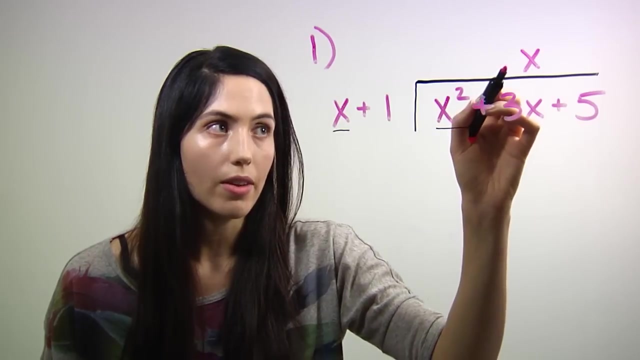 So we put that x up here on top and in line with the 3x term, so that's where it belongs. The next step is to multiply this x by each of these terms and place what you get directly underneath this polynomial. So in this case we have x times x, which gives us x squared. 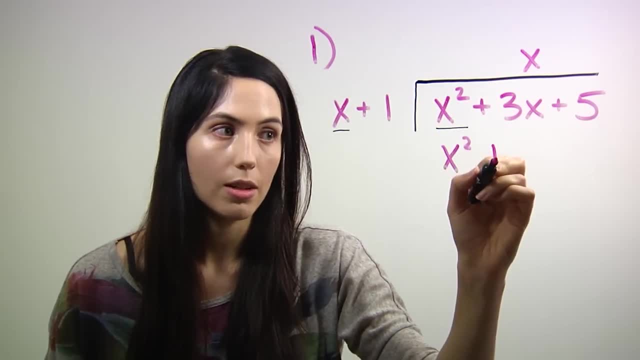 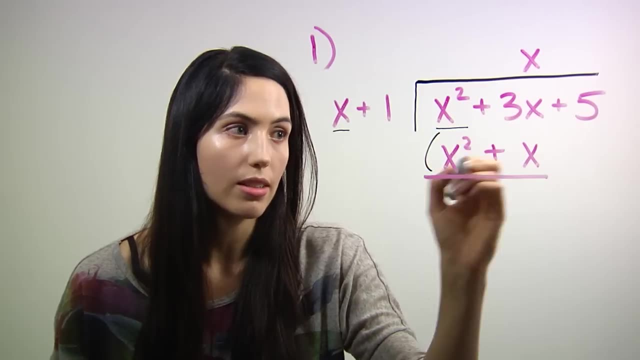 and we have x times x squared, which gives us x squared. and we have x times x squared and we have x times 1, which gives us plus x. Then we want to subtract this line from the first line, so we have x squared plus 3x minus. 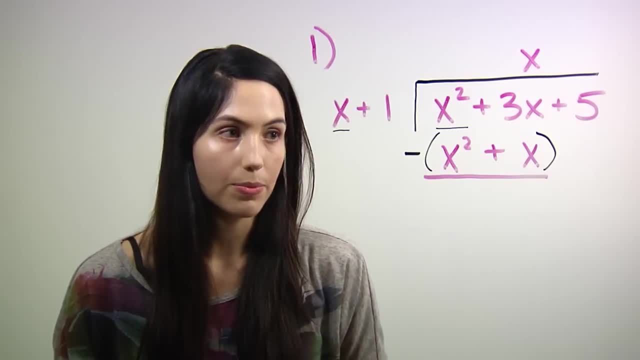 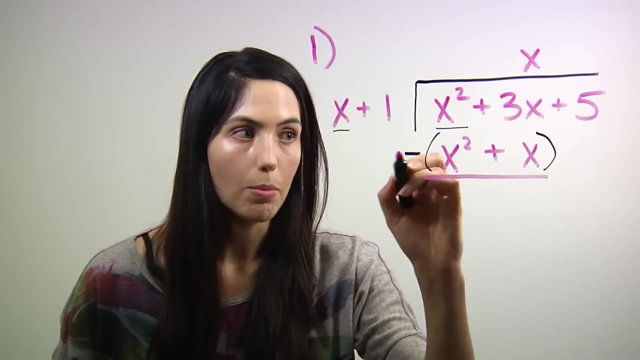 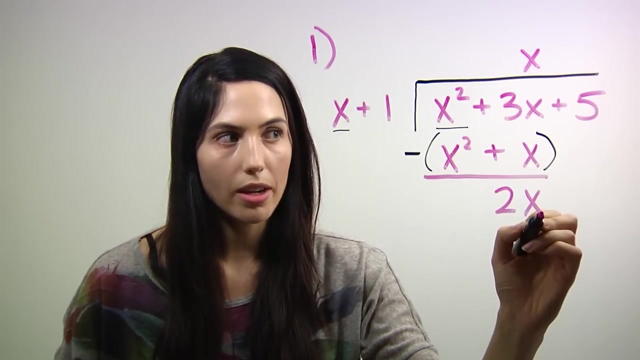 x squared minus x, so we get below 0, nothing here- and we have 3x minus an x, so we actually have 2x down below Now, if you think back to elementary school, when you first did long division at this. 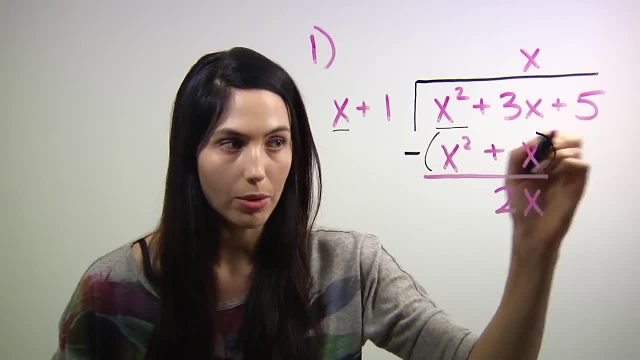 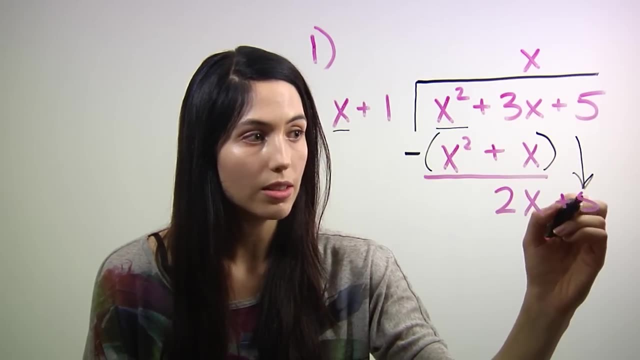 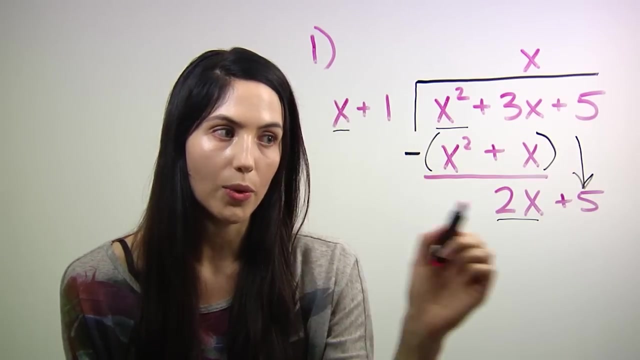 point. we carry down. we bring down this number, the 5, we bring down the next term to this line. so now we ask: how many times does this x go into this 2x, and that's 2 times. 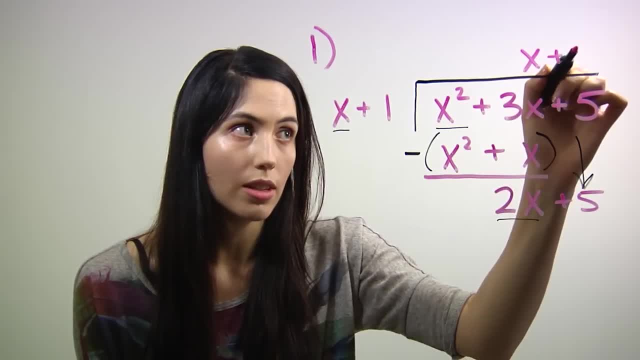 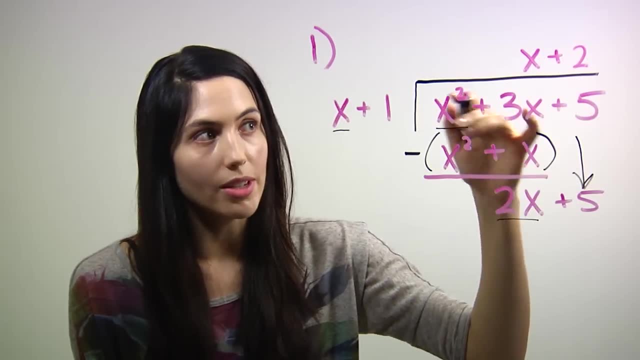 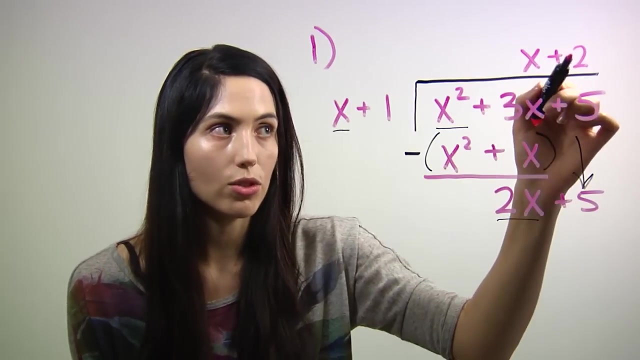 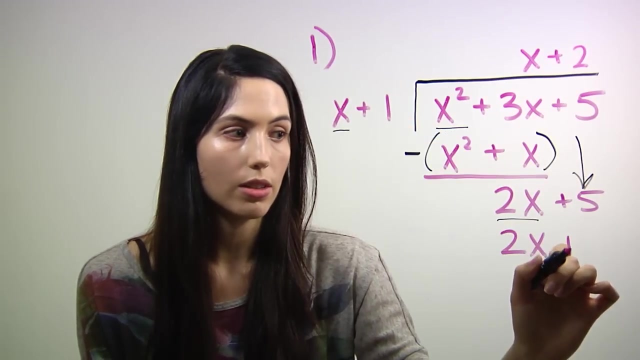 So we write 2 here up top in line with the other number, the other constant. Now let's repeat that first step of multiplying that number, that term by the whole divisor and writing it below. So in this case we have 2 times x and 2 times 1, so plus 2.. 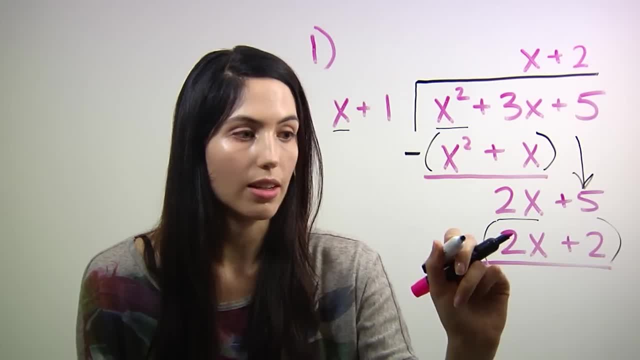 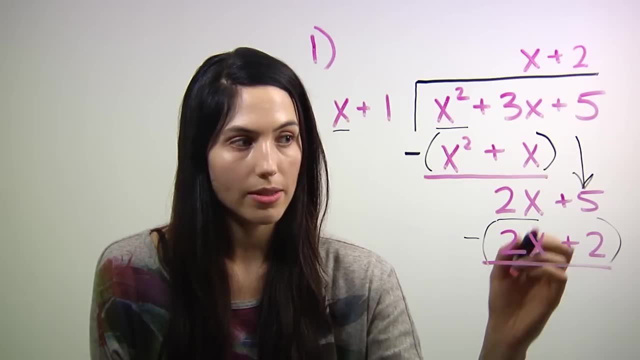 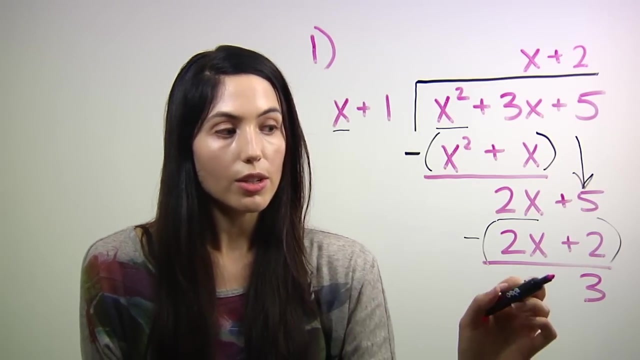 And again, as before, we're going to subtract. We subtract that line from the line above and we get nothing here: 2x minus 2x, and here we have 5 minus 2, so 3.. Now, as a final step, you do need to still ask yourself: does my divisor x plus 1, go? 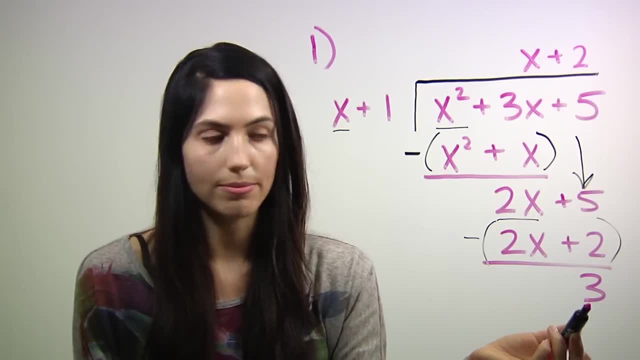 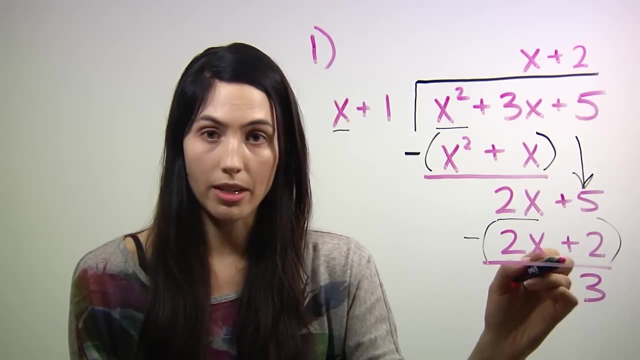 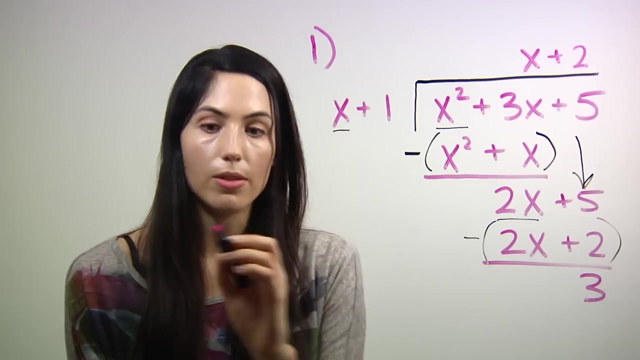 into 3 any more times. And the answer is no, because x plus 1 is a larger polynomial than 3.. So you're done. This is your remainder. So in your class, most likely you're going to want to write the answer as x plus 2 with. 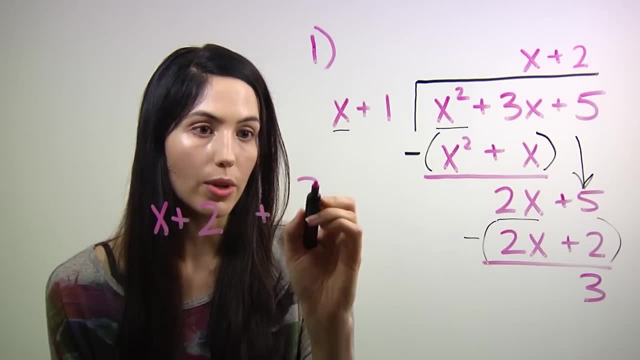 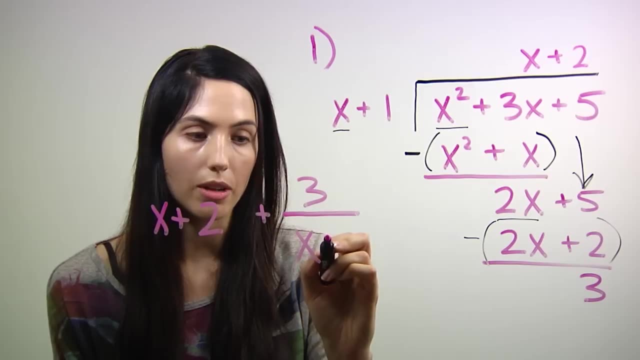 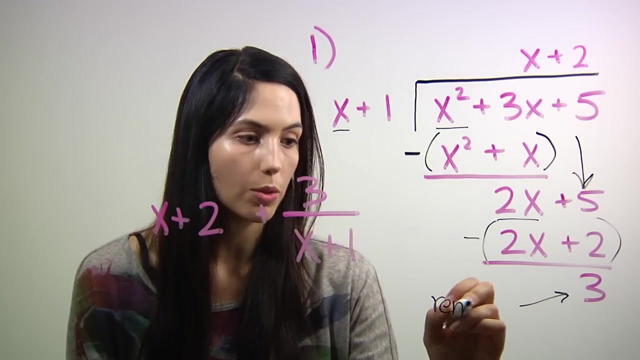 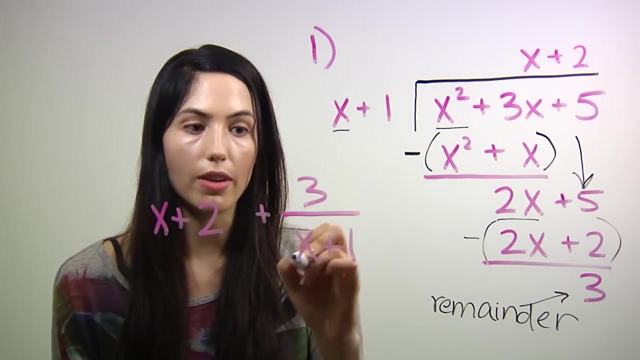 a remainder of 3, and typically you put the remainder over the divisor, So in the bottom we have x plus 1.. So that 3 was your remainder And you always place it in the end over your divisor x plus 1.. 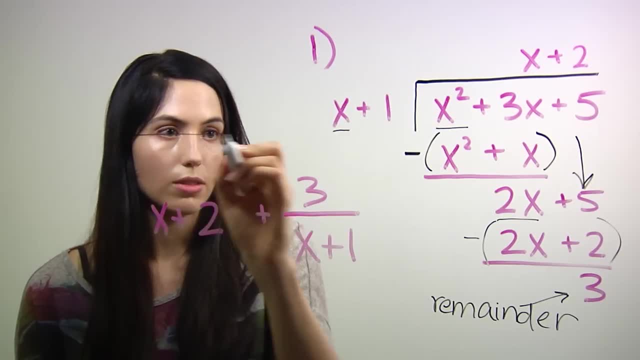 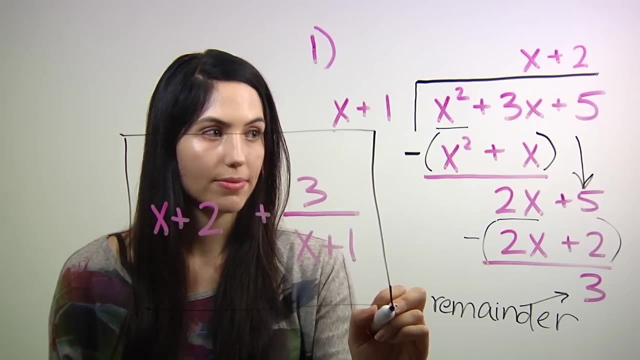 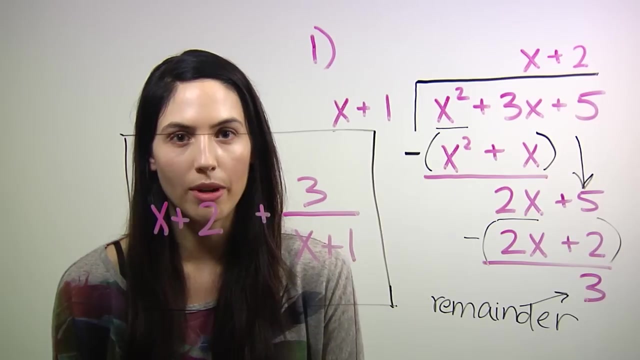 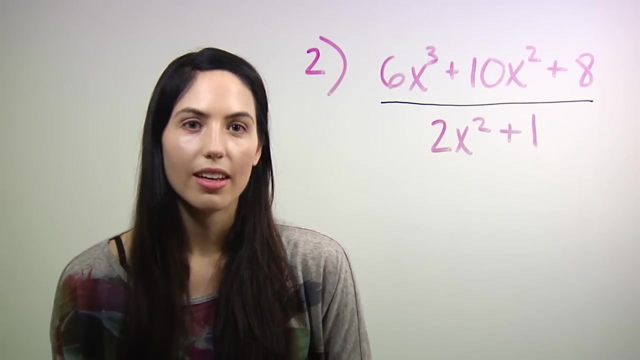 So your final answer is x plus 2 plus 3 over x plus 1.. Okay, so that was fun. That was a simpler, more straightforward version of the long division with polynomial problem. Now let's look at a harder one. Okay, so we're going to rewrite this again in the other division form. 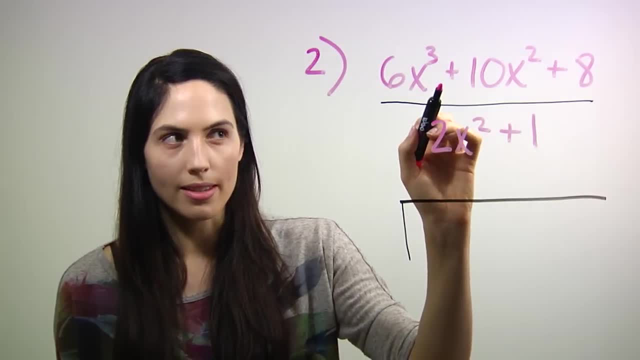 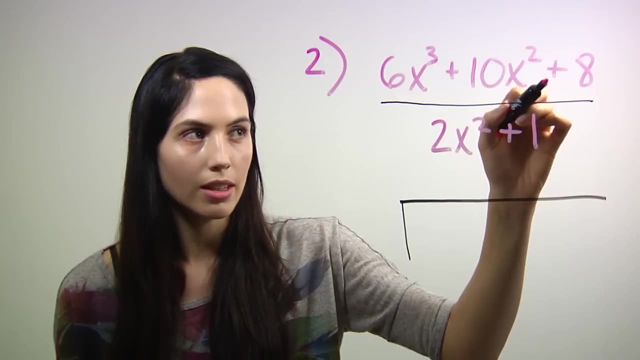 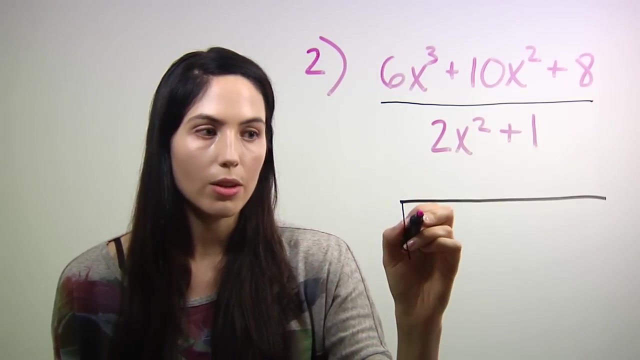 And notice that in this case in that top polynomial there is a term missing. There is no x term, 2x, 1x, So we actually will need to leave a placeholder for it. So let's rewrite this: We have 6x cubed like normal, plus 10x squared. 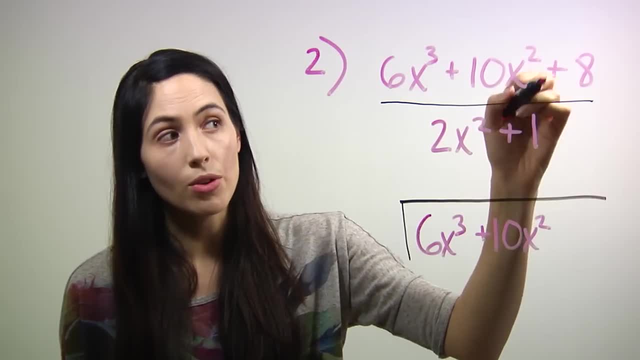 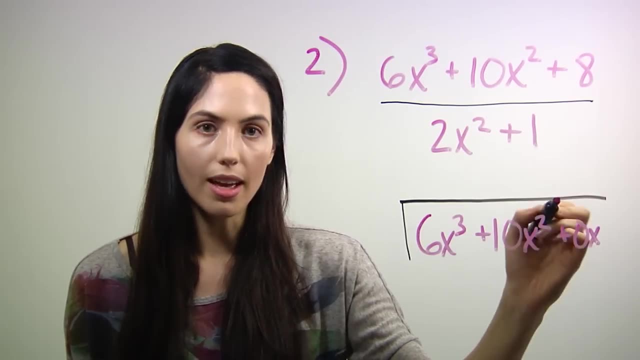 Now, in this place where there's a gap, where there's no x term, we need to write 0x here in the dividend as a placeholder. That's really important that you put that 0x there if there's a gap. 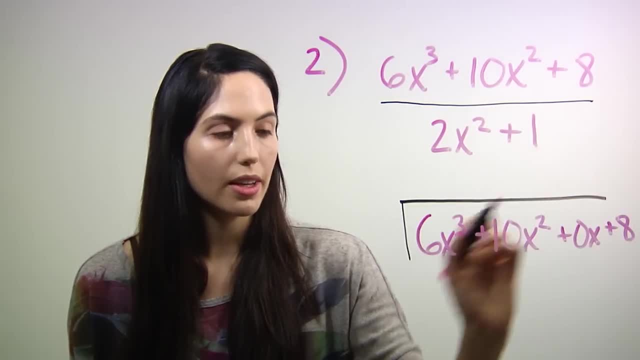 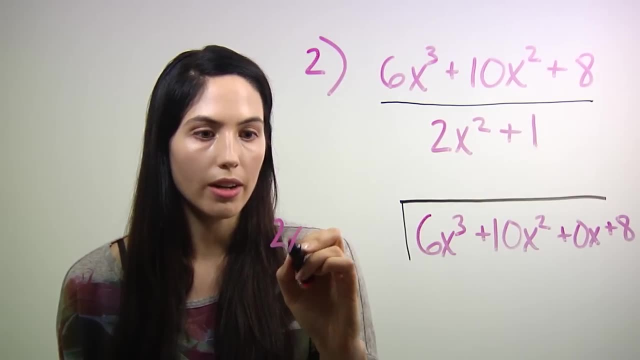 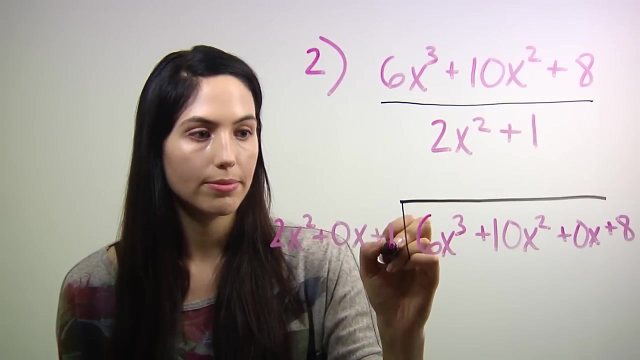 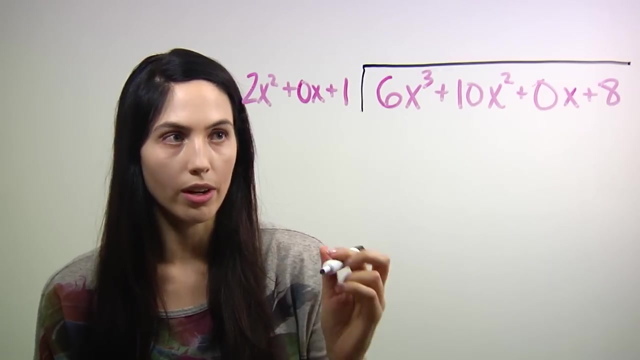 And then plus 8.. And then our divisor in the bottom: 2x squared plus 1.. Same thing. We'll write 2x squared. Notice: there's no x term, So we put 0x plus 1.. Okay, so now that we've rewritten this problem in the normal division form, let's carry out the same steps as before. 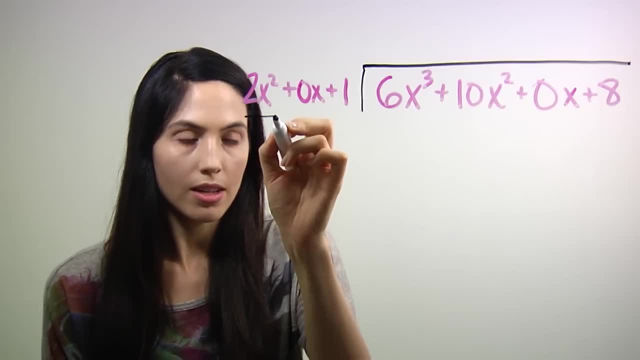 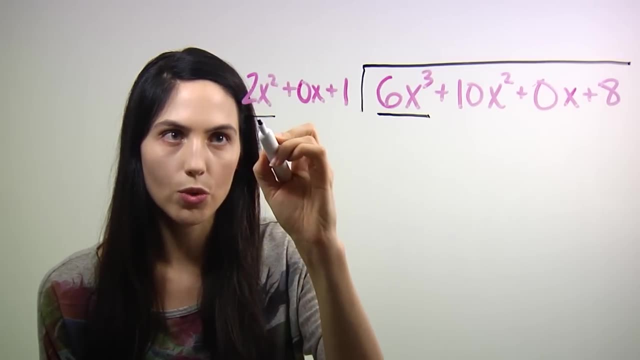 So look at this highest power of x on the left side and the highest power of x underneath And we want to know how many times does that turn out to be? How many times does that term 2x squared go into this term, 6x cubed? 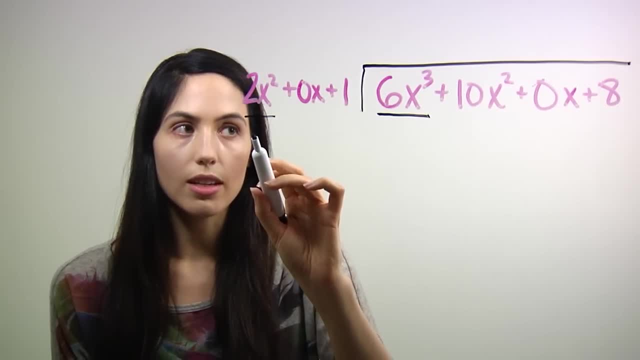 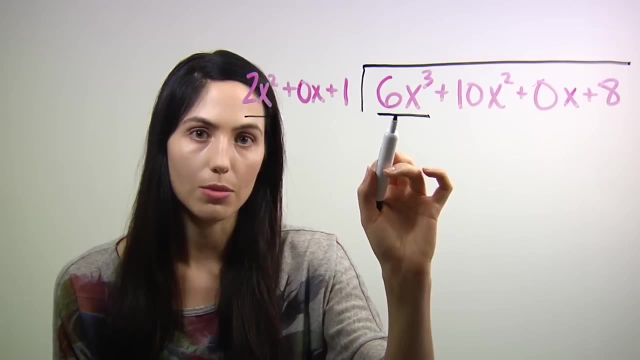 So how many times does 2x squared go into 6x cubed? The answer is 3x, because 3x times 2x squared would give us back 6x cubed. So the 3x we place up here on top. 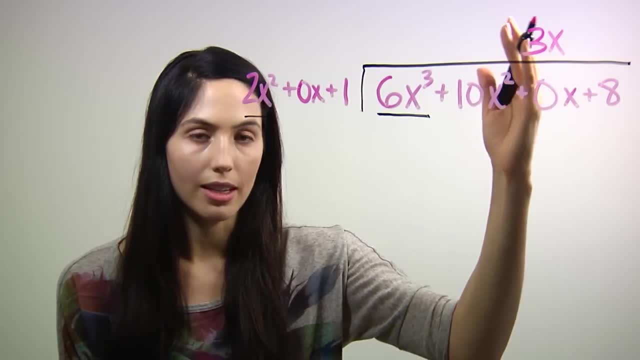 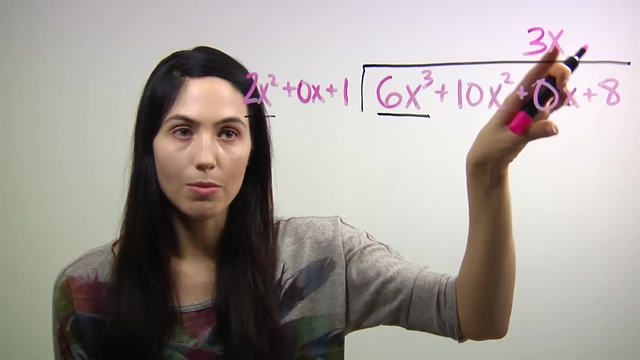 Make sure you place it right above the other x term, in line with the other x term, If you remember this step from before. we're going to multiply that term 3x by each of these in the divisor and write the expression we get underneath. 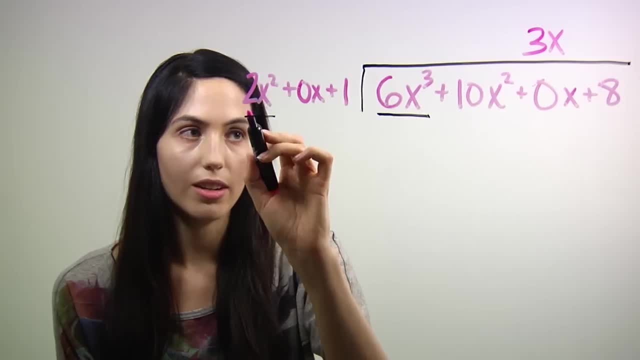 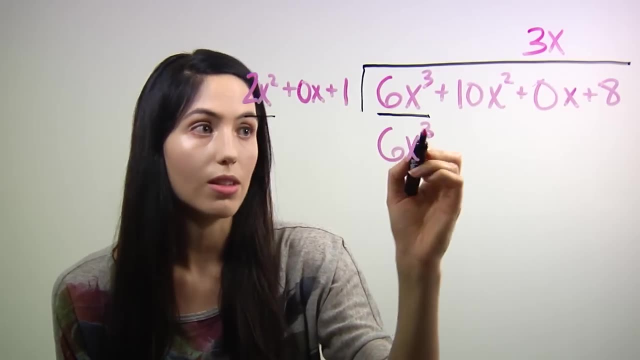 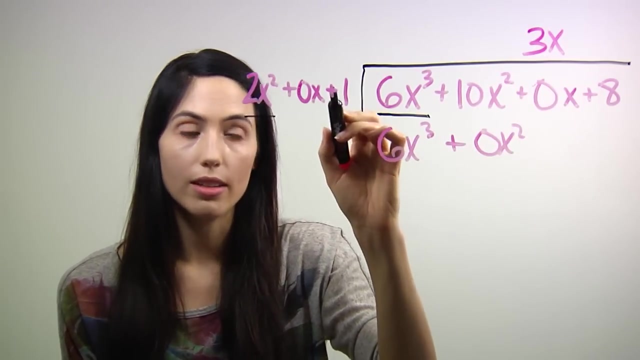 So in this case we have 3x times 2x squared, which gives us 6x cubed. 3x times 0x, which just gives us 0x squared. 3x times 1, which just gives us 3x. 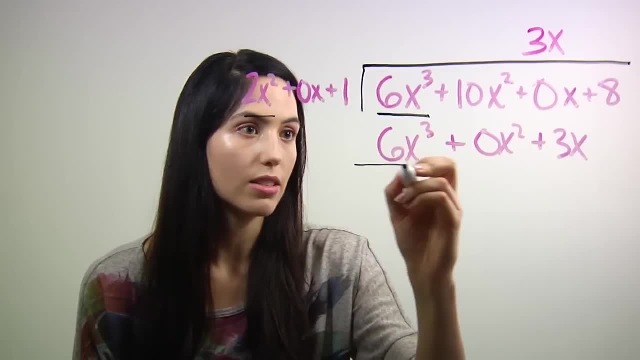 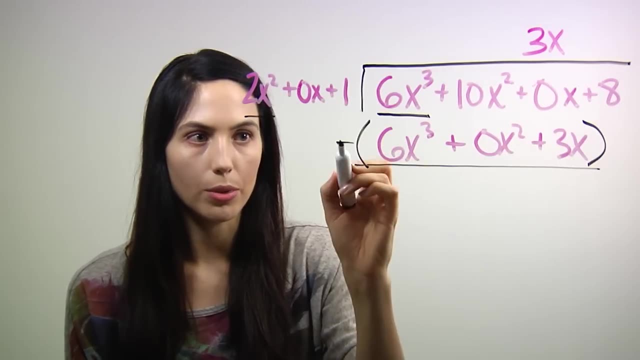 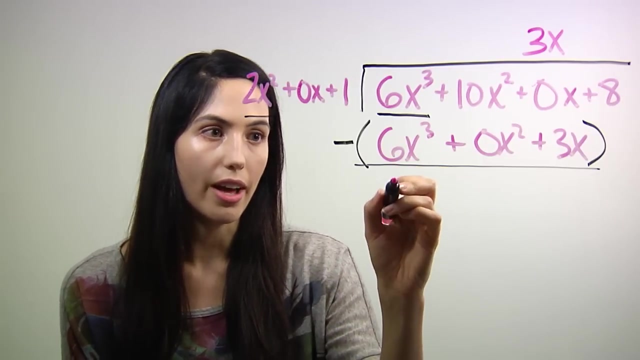 We're going to subtract, so draw your line. We're going to subtract that whole second line. It's important to draw those parentheses and put the overall minus so that you get the signs right. So down below, when we use the subtraction, we'll have nothing here. 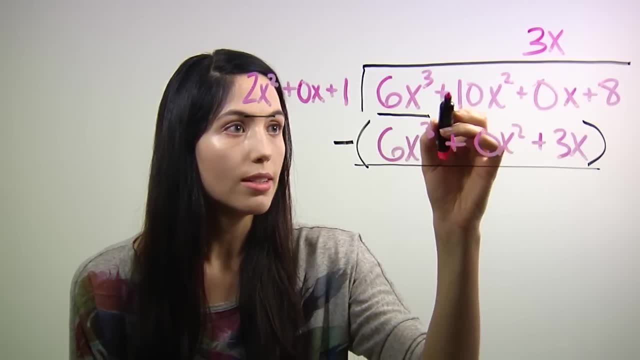 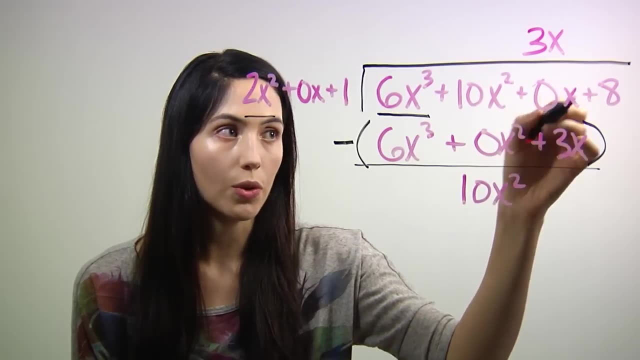 6x cubed minus 6x cubed is 0.. 10x squared minus 0x squared leaves us with still 10x squared: 0x. 0x. 0x minus 3x is minus 3x. 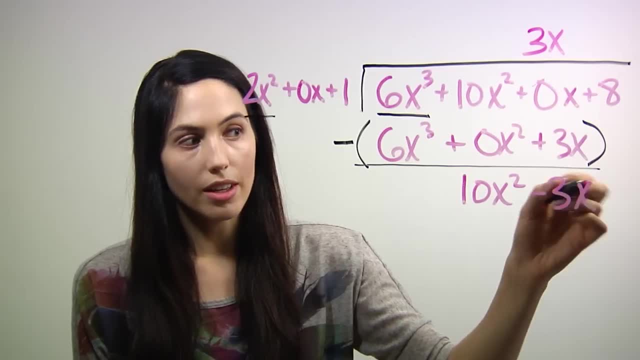 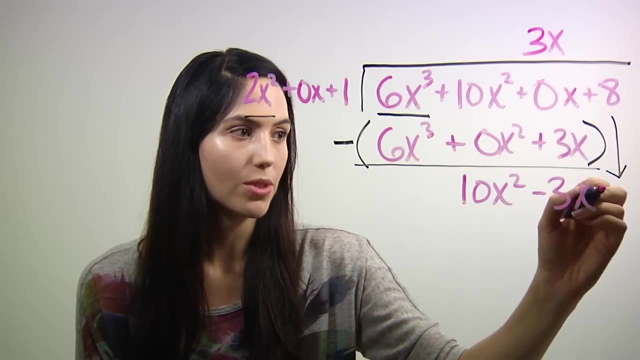 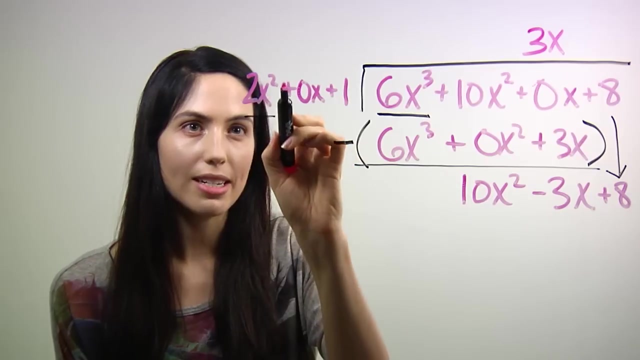 Now remember your long division steps. At the end of this, we want to carry down this number, carry down one more term So we have a plus 8 at the end. Now, final step in the process: how many times does this biggest term in the divisor 2x squared? 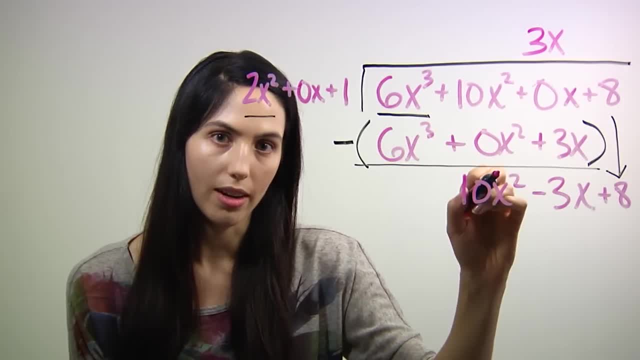 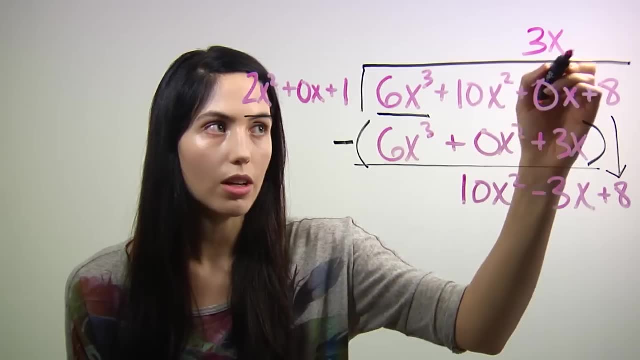 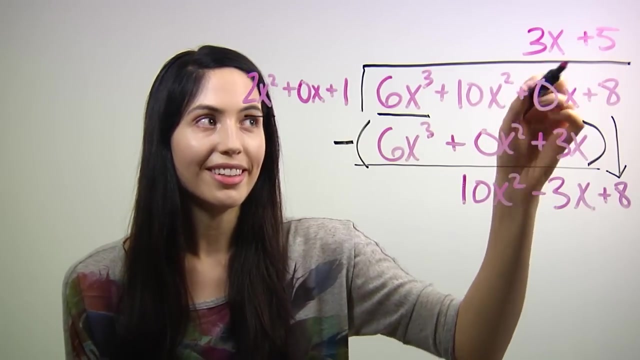 go into this term 10x squared, and the answer is 5, because 5 times 2x squared is 10x squared. So 5 we place up here right above the other constant 8.. Now multiplication step. 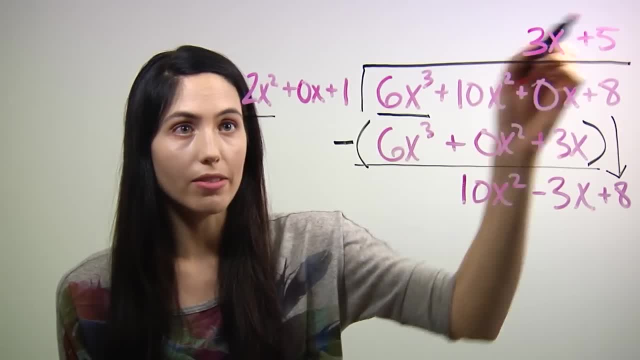 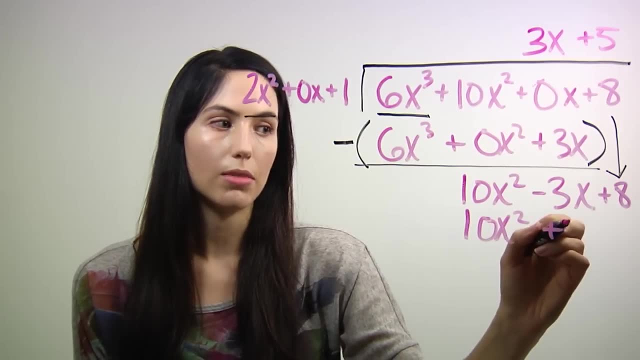 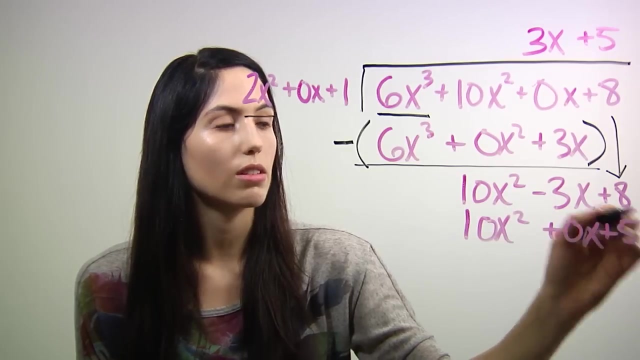 So we're repeating the steps at this point. 5 times 2x squared is 10x squared, 5 times 0x. 0x, 0 times. anything is 0.. 5 times 1 is 5.. 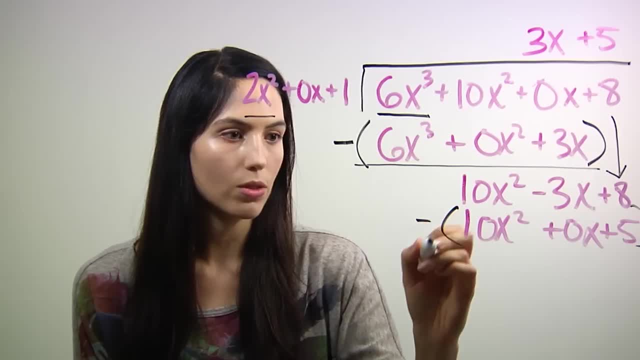 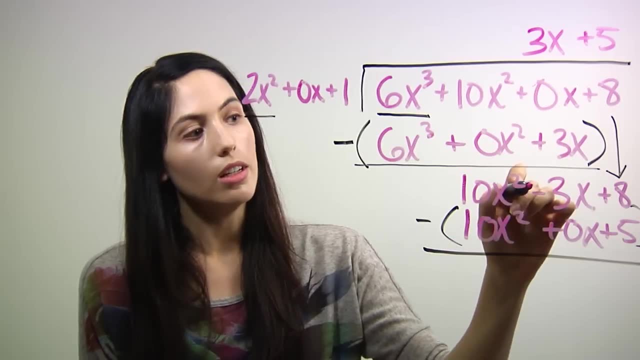 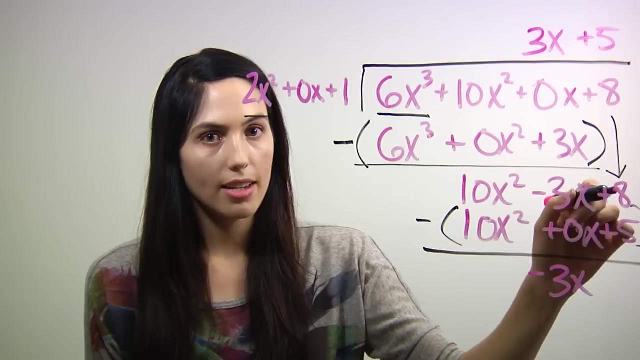 Final subtraction: Draw your parentheses. Draw your subtraction line Down below. we have nothing here. 10x squared minus 10x squared Negative: 3x minus 0x is negative. 3x 8 minus 5 is plus 3.. 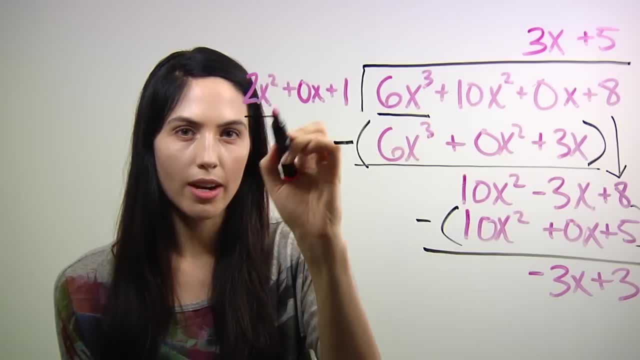 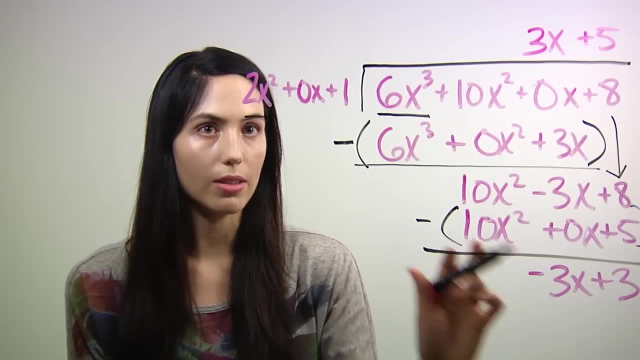 So now ask yourself: does 2x squared in the divisor go into negative 3x any more times? And the answer is no, You're done, because this term is larger than that term and you can't fit it inside it anymore.